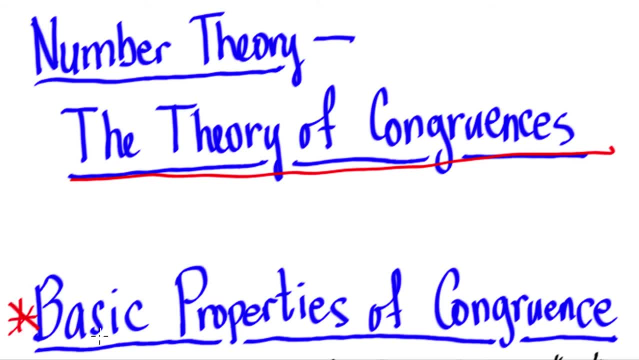 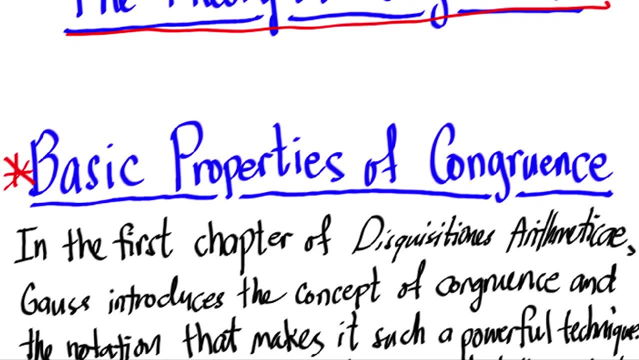 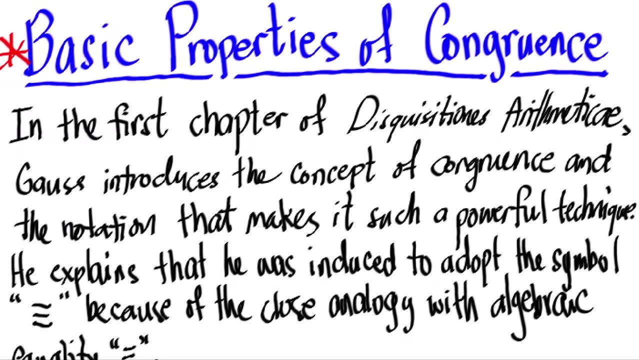 and most foremost topic, which is the basic properties of congruences. So we're going to go back a little bit in history. Hopefully you watched the first video about concerning Gauss. okay, our princeps mathematicorum, our prince of mathematicians, Gauss. So in the first chapter, 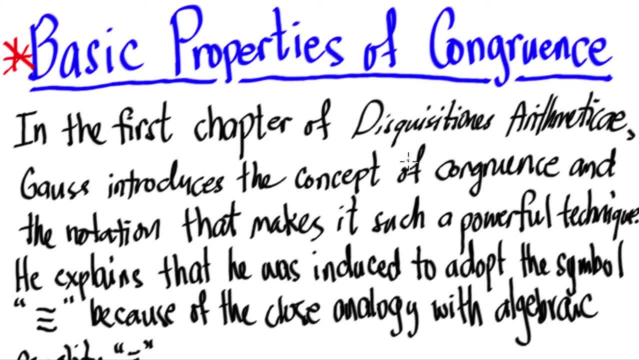 of his famous book and most magnificent book, Disquestiones Arithmeticae, Gauss introduces the concept of congruence and the notation that makes it such a very powerful technique. He explains that he induces congruence. He explains that he induces congruence. He explains that he 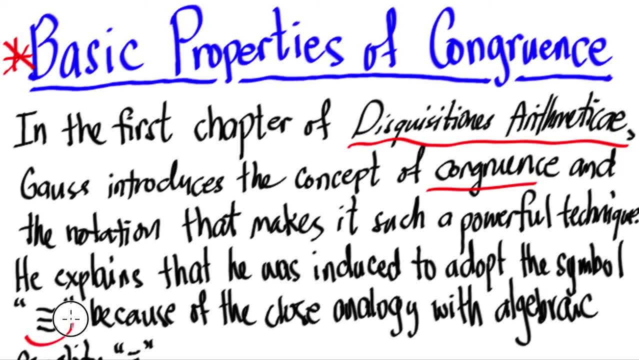 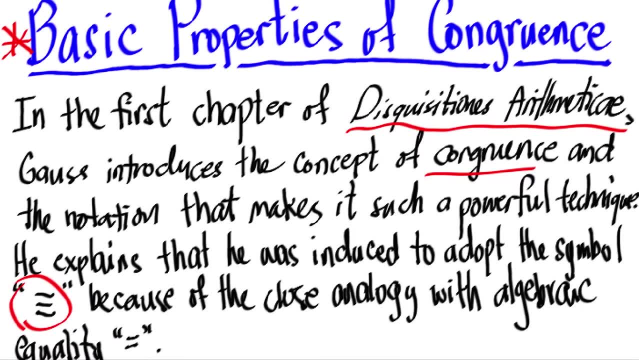 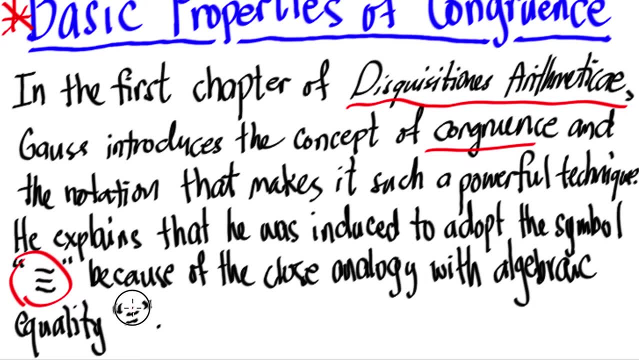 or he was induced to adopt the symbol, this one, the triple parallel lines, because of the close analogy of it with the algebraic equality, or simply as the equal sign. Okay, so we can remember the equal sign and know that we are aware of it. The equal signs are only composed of two parallel lines. 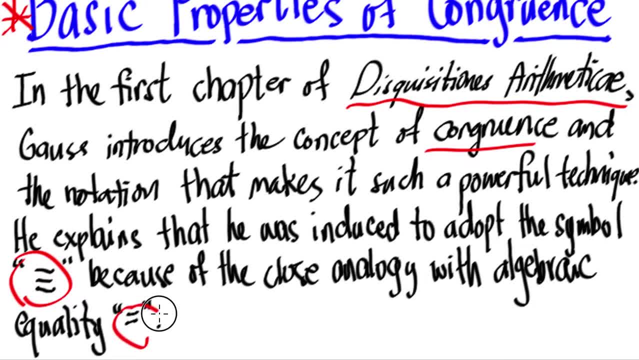 while the symbol for congruence is composed of three parallel lines. okay, here, Okay, so let me explain this a little bit more. So, Gauss, he says that if a number n measures the difference between two numbers, a and b, okay, then a and b are said to be congruent with respect to the 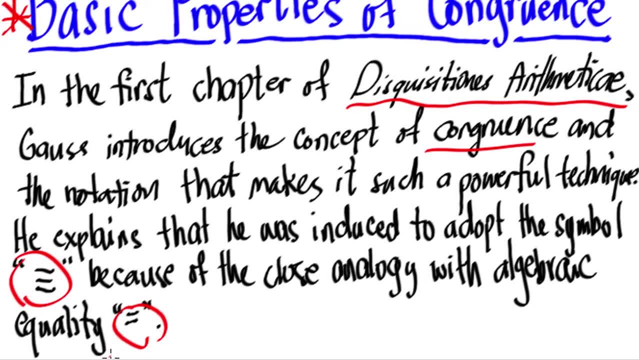 modulo n. Okay, we call that modulo n. If not, we call a and b to be incongruent. So let's put this in a formal way, shall we? So let's put this in a formal mathematical definition. So here, let's. 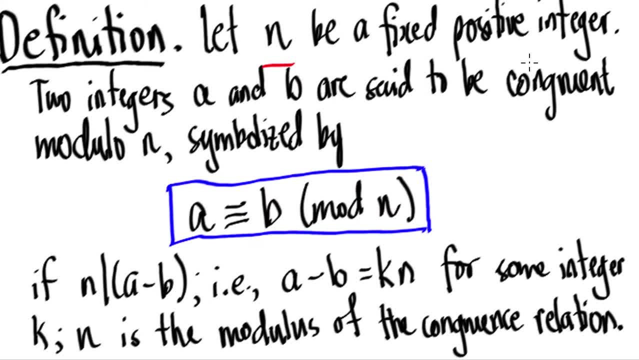 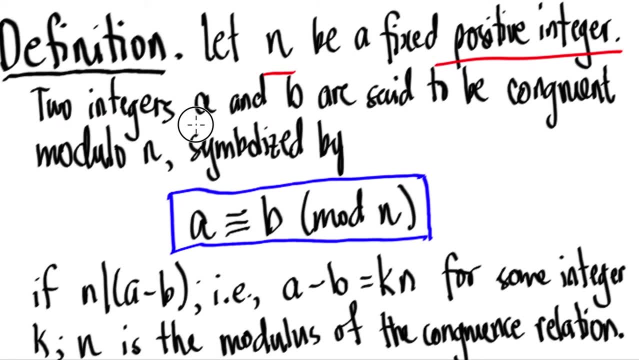 define a, let n B a fixed positive integer. Okay, it's a positive integer, Fixed positive integer n. And then two integers, a and b, are said to be congruent, modulo n, symbolized as this: Okay, a is congruent to b. We read this as: a is congruent to b, modulo n: Okay again. 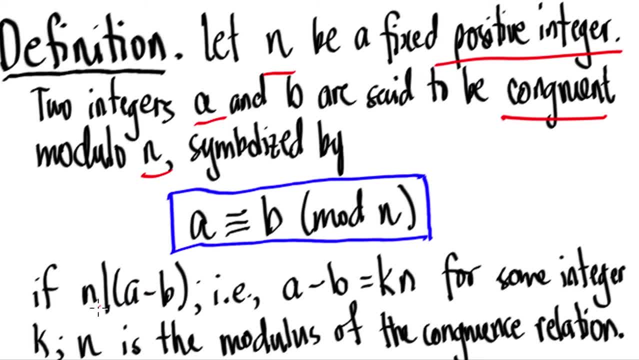 a is congruent to b modulo n. if n divides a and b or divides a minus b, rather Okay. this is a and b. N divides the difference of a minus b, That is, a minus b is equal to n times this sum integer k. 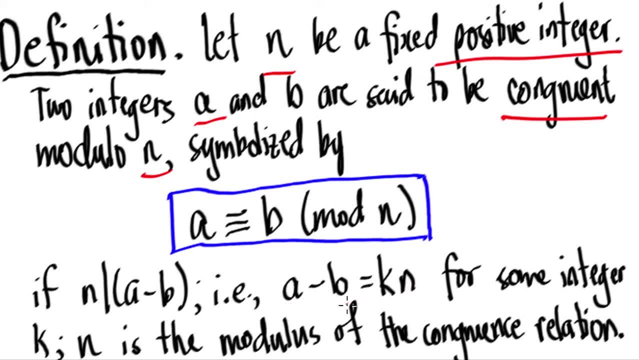 because n is said to be a factor of a minus b. N is what we call the modulus of the congruence relation, or simply the modulo. Okay, it's like the clock In the clock arithmetic: it's the one that gets the remainder and then gives you the value of a. Anyway, 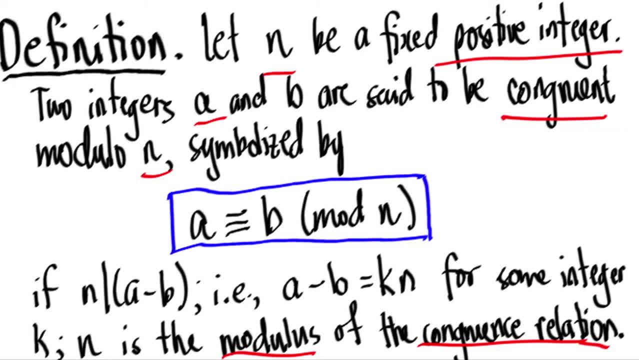 I'm going to illustrate that to further, to clearly explain that one. Anyways, just put in mind that a is congruent to b modulo n if n divides the difference of a minus b, or, conversely, if n divides a and b. So therefore we can say, therefore, that a is congruent to b mod n. 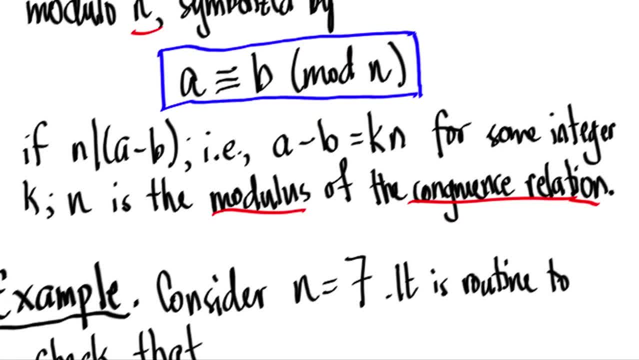 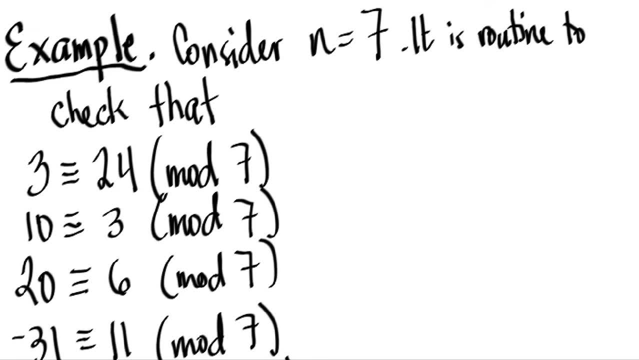 So, to cite some examples, shall we say: anyways, the n again is what we call the modulus of the congruence. Okay, so, as for example: so let's have, let's cite some examples. So consider your modulo n to be equal to 7, for example, Let's have, n equals 7.. So it is. 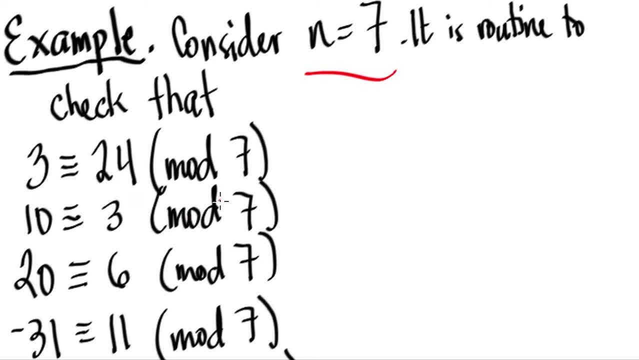 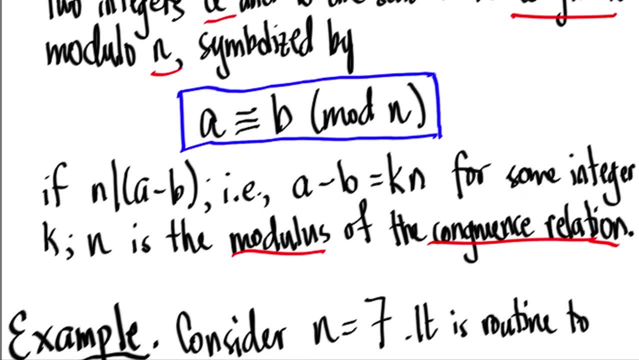 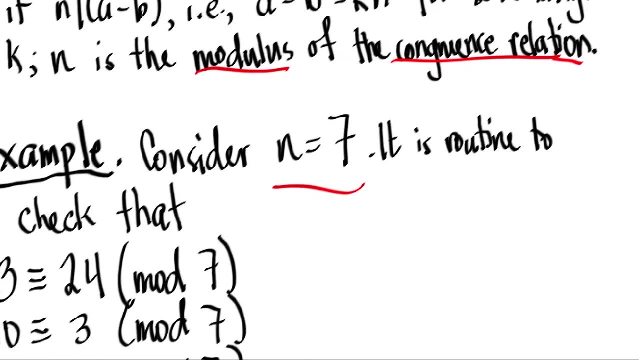 routine to check that 3 is congruent to 24 modulo 7.. Why is that so? Okay, let's recall the definition going up here. We say that a is congruent to b modulo n if n divides a minus b. So let's apply. 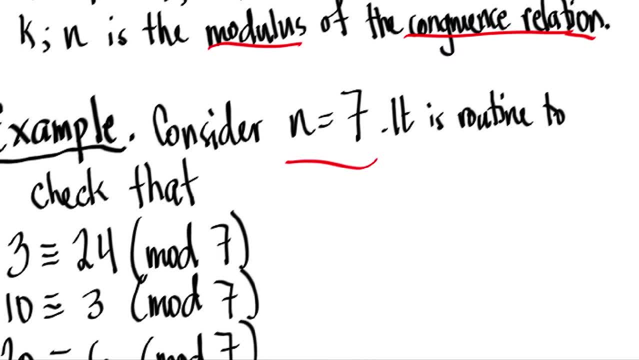 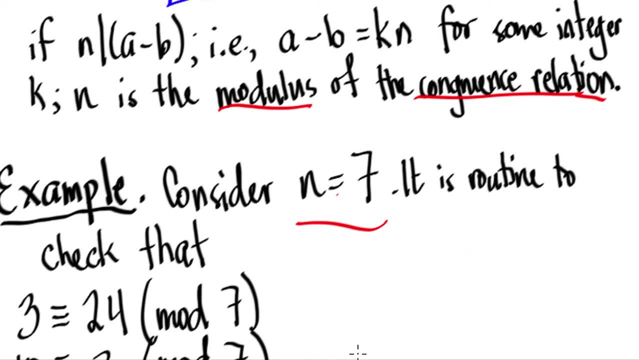 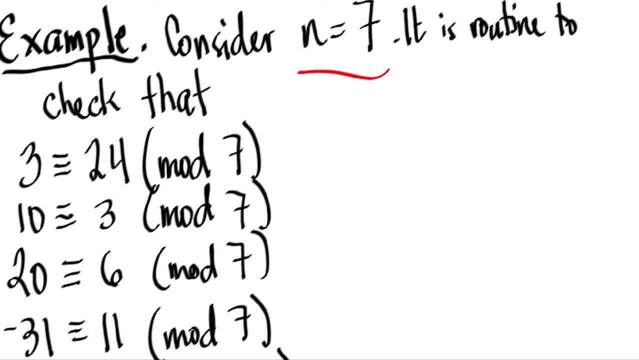 that here. Anyways, let's show the definition first. Okay, if n divides the difference of a minus b, therefore a is congruent to b mod n, So let's apply it here, Okay. Okay, why is this so? Why is 3 is congruent to 24 mod 7? Because 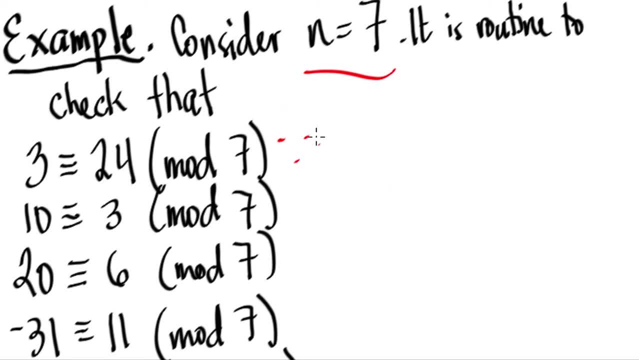 shall we put it here? Because, Okay, anyways, this is the symbol for, because, Remember, this is the symbol for. therefore, It's a triangle, triangular dot. If you reverse a triangle, so you'll have the symbol for, because So 3 is congruent to 24 mod 7, because 3 minus 24.. 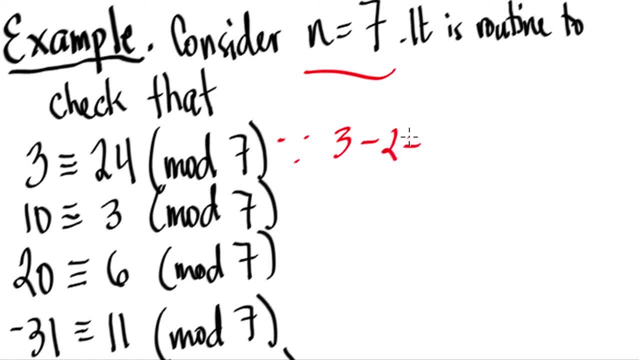 So what is 3 minus 24?? So 3 minus 24, we know of as negative 21,. right, That's understood to say that 3 minus 24 is negative 21.. And we know negative 21 as a multiple of 7.. Okay, 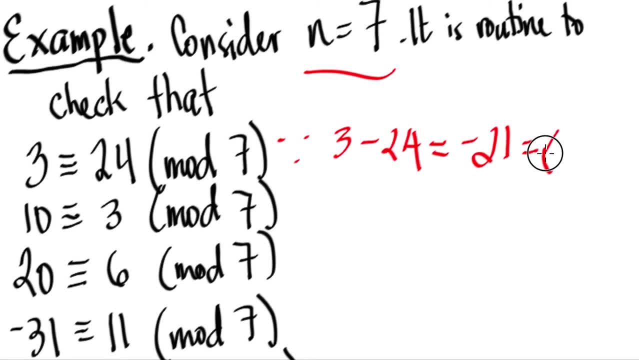 basically, that is negative 3.. It is negative 3 times 7.. Negative 3 times 7.. Okay so, negative 21 is negative 3 times 7.. Next let's move on to the next number. So we see that 10 is congruent to 3 modulo 7,. 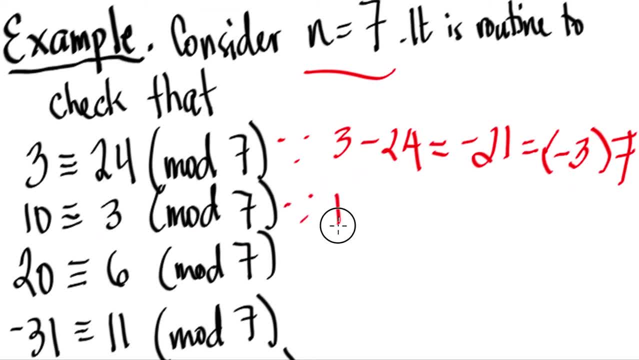 Why is that so? Because 10 minus 3 is equal to 7.. We say that it's equal to 7, and we know 7 is a multiple of 7, because 1 times 7 is 7.. So that's true. Therefore, that's true, It's correct though. 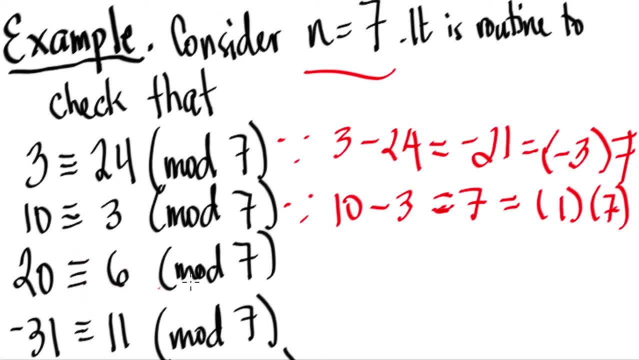 Okay, how about this? 20 is congruent to 6 modulo 7 because- let's try it again- 20 minus 6 is equal to 14, and 14 we know of as 2 times 7.. So, therefore, 20 is indeed congruent to 6 with respect to the modulo, which is 7.. 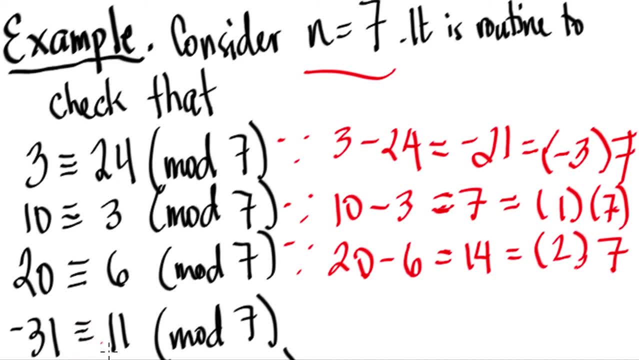 Okay, next up, we have negative 31.. It's congruent. It's congruent to 11 mod 7.. Why is that? Let's check That's indeed true. So we have negative 31 minus 11.. 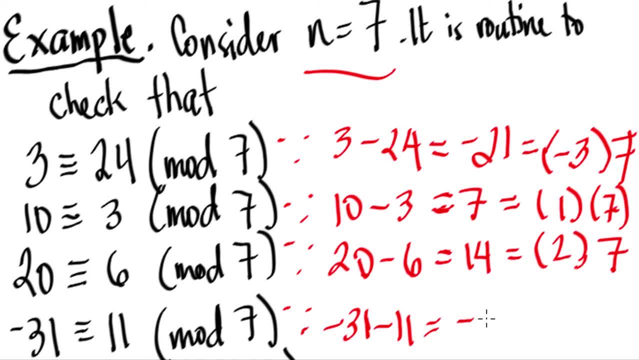 What do we have? So they're both negative, So we'll have negative 42.. Okay, which is 42 or negative? 42 is indeed a multiple of 7, because negative 6 times 7 is equal to 7.. 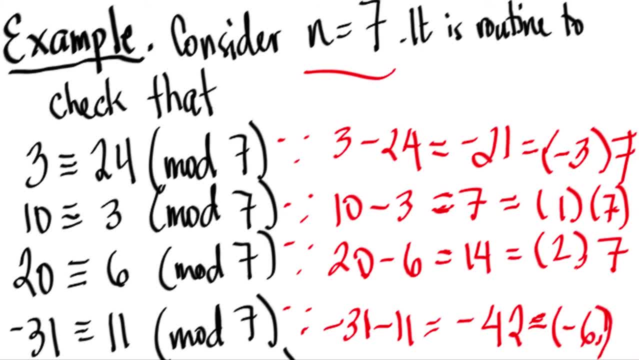 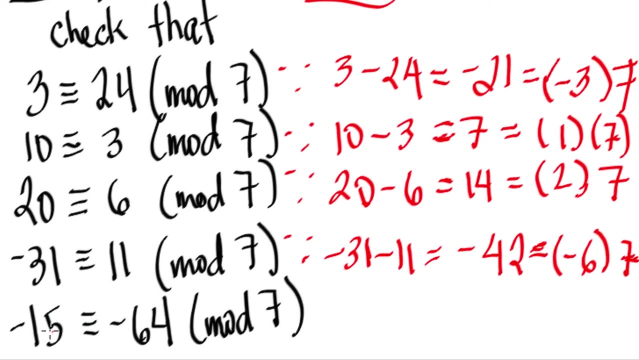 So we have negative 42. Again, negative 6 times 7 is equal to negative 42.. Okay, now let's move on to the next example. This next example is a little bit challenging here. So what we have is negative 15, or rather, negative 15 is congruent to negative 64 modulo 7.. 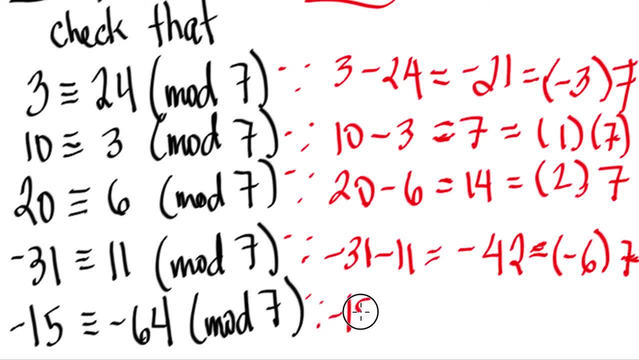 Why is that? Because let's check negative 15 minus negative 64, okay, is going to give us what number. So negative 15 minus 64 is going to give us negative or positive, since this is going to become positive right. 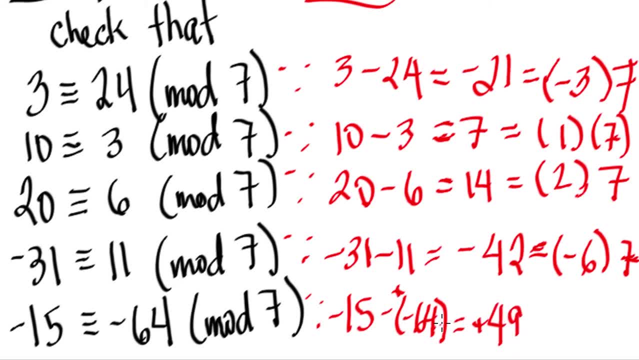 Positive 49.. Okay, so it's like 64 minus 15, right, 64 minus 15.. It's positive 49.. And we know positive 49 as 7 squared, which is clearly 7 times 7.. 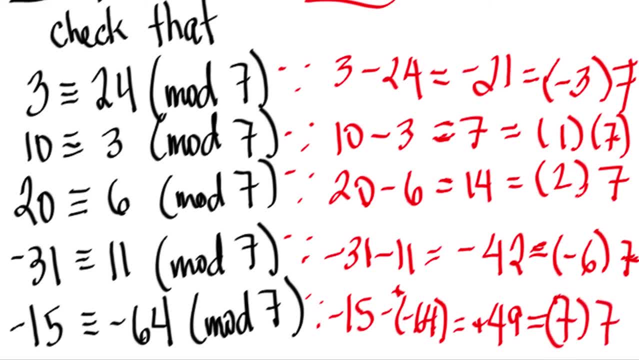 7 times 7.. Okay, so that is the concept of the congruence, the theory of congruence. We have this modulo. Now maybe you are thinking: what's the purpose of this? Okay, where do we apply this in our everyday life? 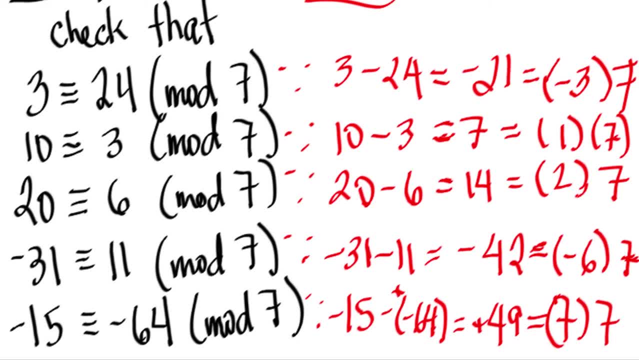 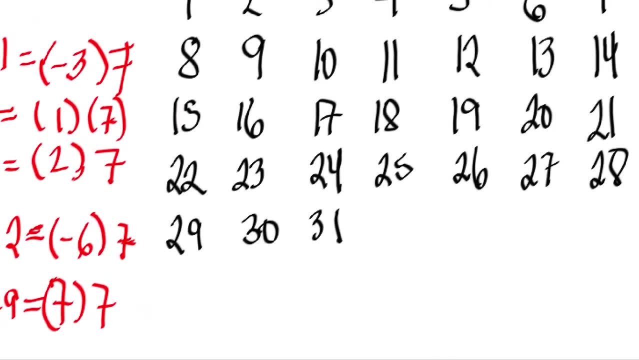 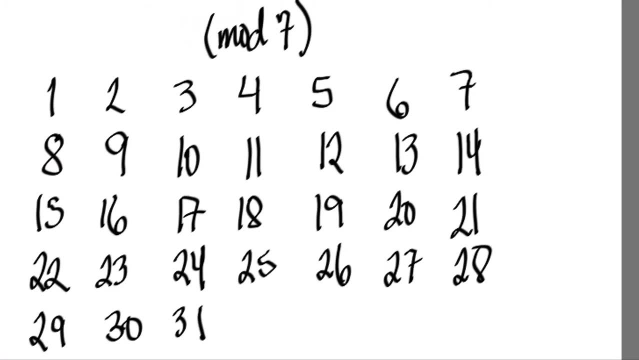 Why do we need to study this? I'll give you one. I'll cite you one example wherein we're going to apply this kind of thinking. So imagine again, we're going to still use the modulo 7.. And imagine that we are talking about- okay, imagine we are talking about- dates. 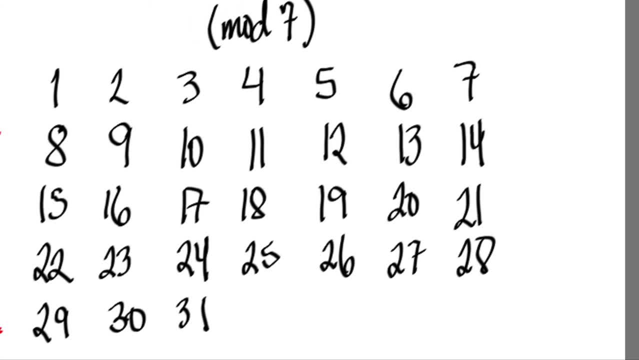 Try to look at your calendars, for example. This is mod 7.. When you say mod 7, when we say 1,, 2,, 3,, 4,, 5,, 6,, 7, okay, after we have 8,, we say that 8, okay is congruent to 1.. 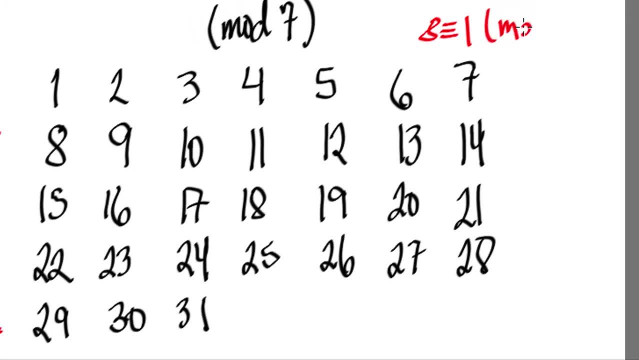 1. Mod 7. Why is that so? So you can try to verify. because 8 minus 1 is equal to 7, which is 1 times 7.. Indeed, they are equal, They're congruent, shall we say. 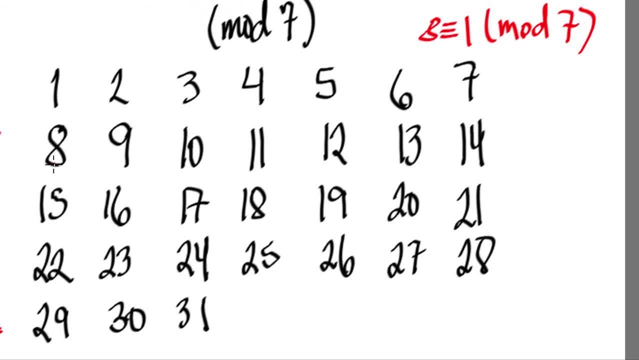 How about this? 15 is congruent to 8.. We can check that. 15 minus 8 is 7.. 15 minus 1 is 14, right? How about this? 22 is congruent to 15.. 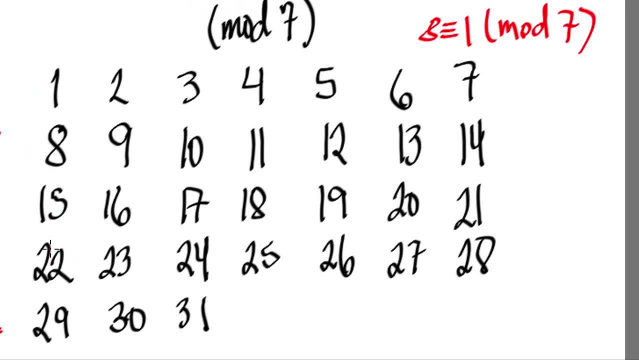 Which is congruent to 8.. Which is congruent to 1,? right, Because 22 minus 1 is 21.. 28 minus, rather, 22 minus 8, is 14.. 22 minus 15 is 7.. 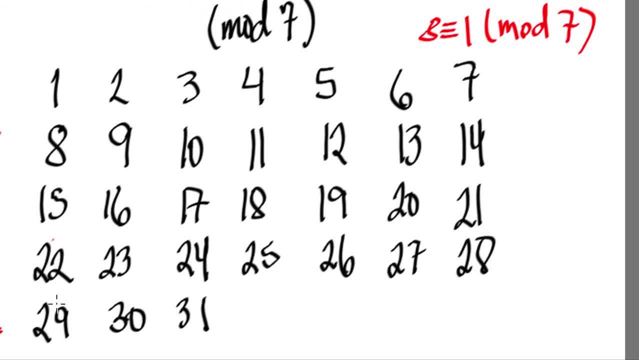 So, meaning we can say that all of these numbers here- 1,, 8,, 15,, 22, and 29,- are all congruent with respect to the modulo 7.. Okay, with respect to the modulo 7.. 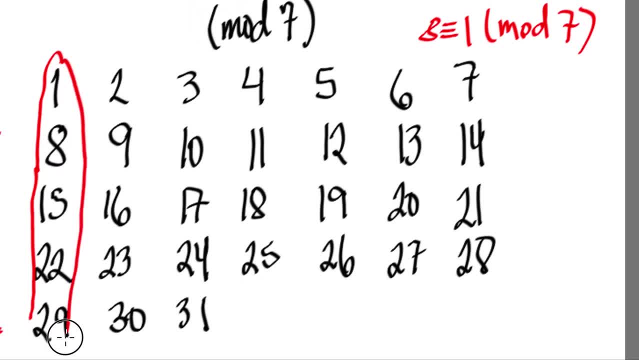 They are all congruent. Okay, They are all congruent With respect to the modulo 7.. Okay, So likewise we can think of that here in our second part. 2 is congruent to 9.. Why is that? 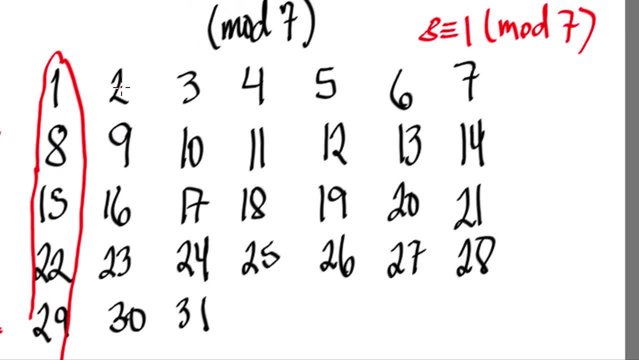 Because 9,, or rather 2 minus 9, is negative 7.. Which is which makes it congruent to- or, yeah, congruent to 7.. Congruent to 2 in respect to 7.. 16 is congruent to 2.. 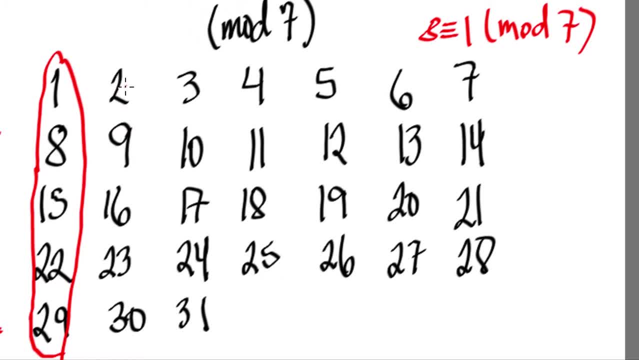 Okay, Because 16 minus 2 is 14.. 23 is congruent to 2, because 23 minus 2 is 21,, and so on, And you can apply that in all of these. Let's try a random one. 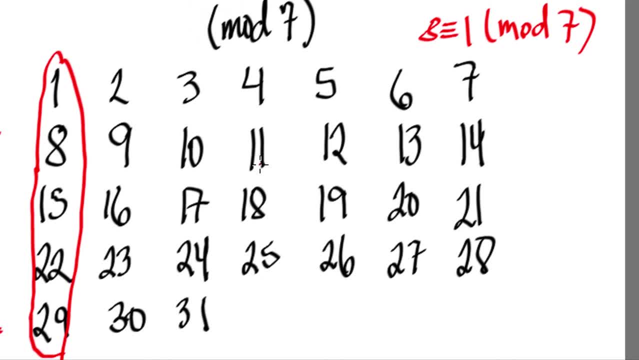 Say, 18 is congruent to 11.. Why? Because 18 minus 11 is 7.. Another one: 27, is congruent to 13.. Why? Because 27 minus 13 is 14.. 21 is congruent to 7.. 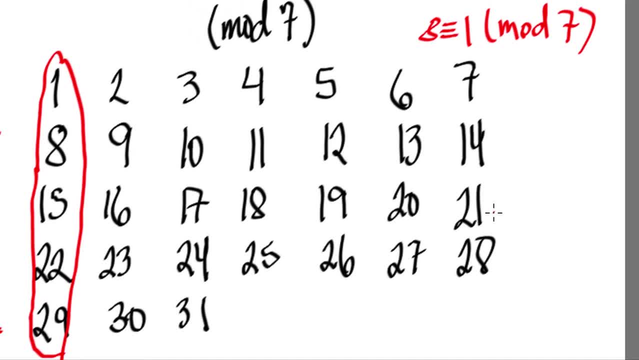 This is trivial because these are multiples of 7.. So they are, of course, congruent to each other, but you can try, you can see that in modular arithmetic, all these numbers here- okay, everything right here, okay, everything right here. okay, all the numbers, all the numbers here, everything here- are all congruent. okay, these numbers are all congruent, okay. meaning in short: yeah, they're not specifically equal, but they're all congruent. 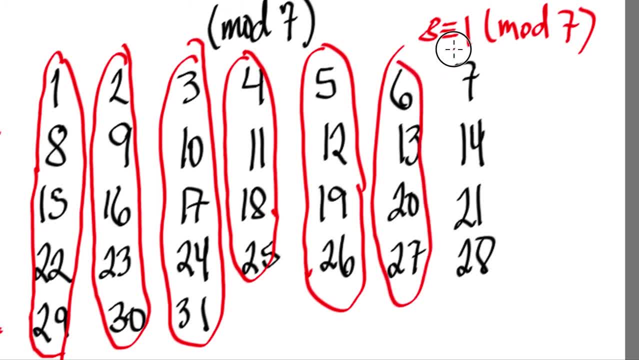 But they are equivalent or they're congruent. We call this congruent or equivalent classes. okay, We call them the equivalent classes or, specifically, they are in congruence with the class modulo 7, or class modulo n, whatever that n is. 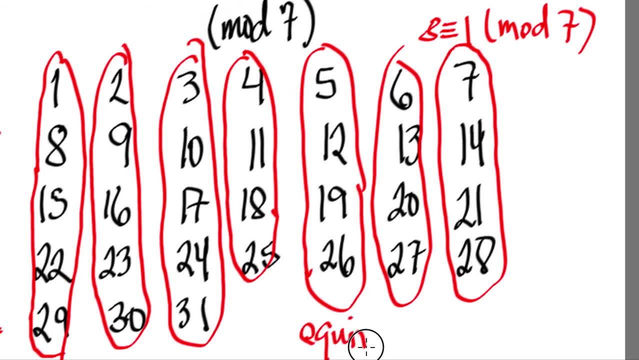 So we call them equivalent classes, Equivalent classes. So they are classes of numbers in which they are congruent with respect to this n. okay, So how do we apply this in our real life? Try to imagine, let's say, all the ones here are Mondays, okay. 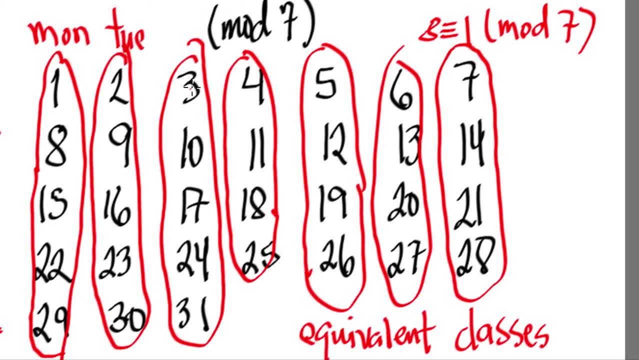 All the twos are Tuesdays. All the congruent with three are Wednesdays: I'll just use W. All the congruent with four is Thursdays: I'll use TH. All congruent with five is Fridays. F- I'll use F. 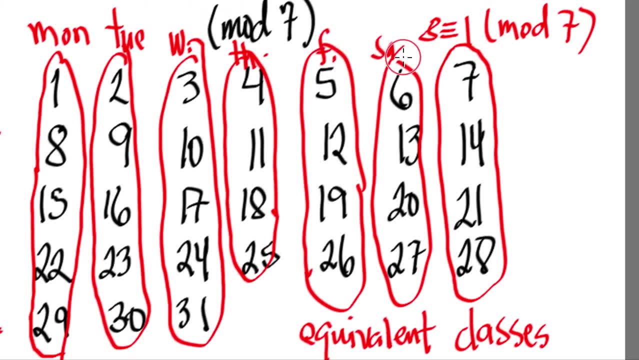 All congruent with six is Saturday, And all that is congruent with seven is Sundays. Now, if we're going to look at your calendar and try to look at the number in which they are equivalent, okay, They are equivalent with respect to the modulo 7.. 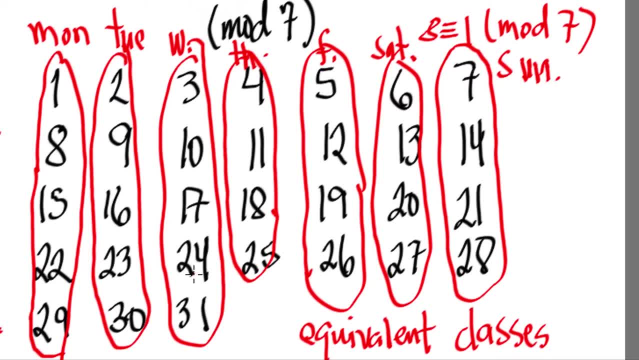 17 and 10.. Okay, 17 and 10 on your calendars are on the same day. Why? Because they are congruent. They are congruent with the number of days in a week, which is mod 7. Meaning they are both. in our case, here, 17 and 10 are both Wednesdays. 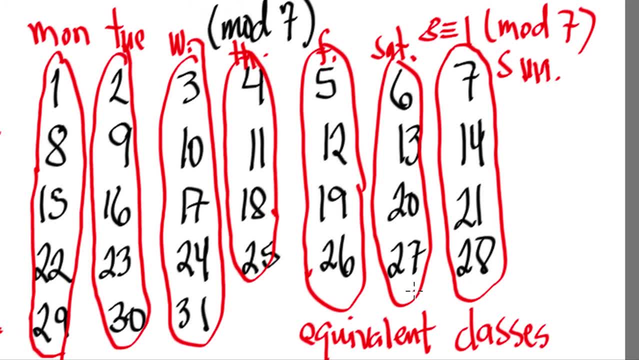 26 and 19 are both Fridays. okay, If you're going to look at your calendars, yes, they are indeed the same. okay, 19 and 12 are congruent. 26 and 19 are congruent. 28 and 21 are congruent. 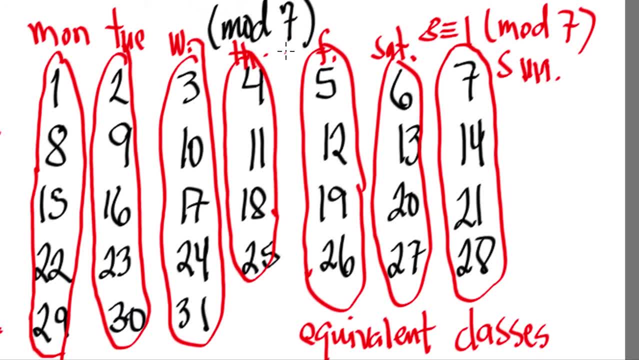 In short, as far as mod 7 is concerned, as far as the number of days are concerned, we go back Going to Sunday, we go back to Monday. Okay, 1, 2,, 3,, 4,, 5, 6, 7.. 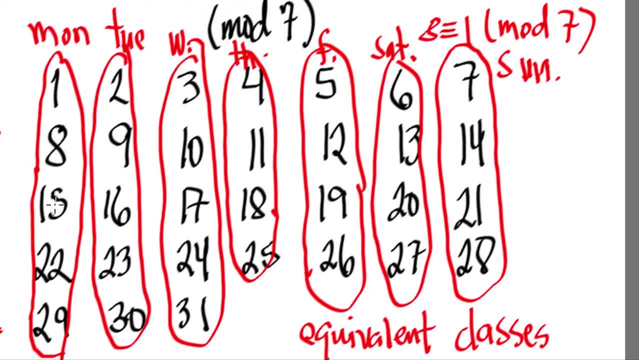 Go back to Monday: 8,, 9,, 10,, 11,, 12,, 13,, 14.. We go back to Monday And then all the numbers here which is equivalent, which are in a single class of equivalents. 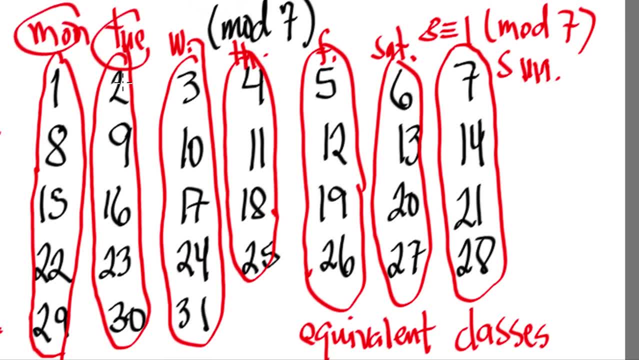 mod 7, are all on the same day, All the same day. All the numbers here are on the same day, All the numbers here are on the same day, and likewise. Okay, Okay. So that's one application of Modular arithmetic. 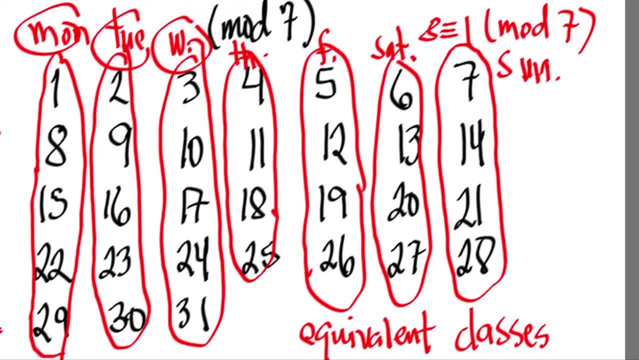 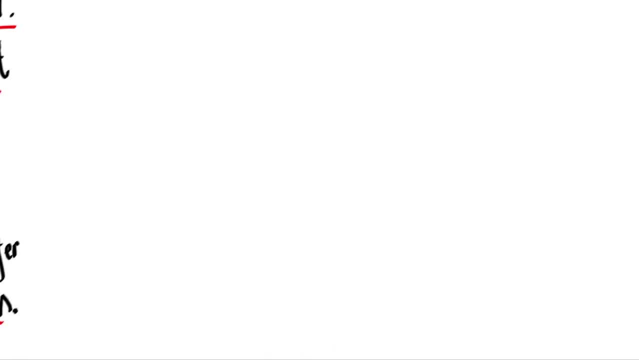 Some call this modular arithmetic or clock arithmetic. Why is it called clock arithmetic, by the way? Because this can be applied in clocks. actually, Just try to look at your clock at home. I'm going to say, I'm going to write a circle, if this is qualified to be a circle. 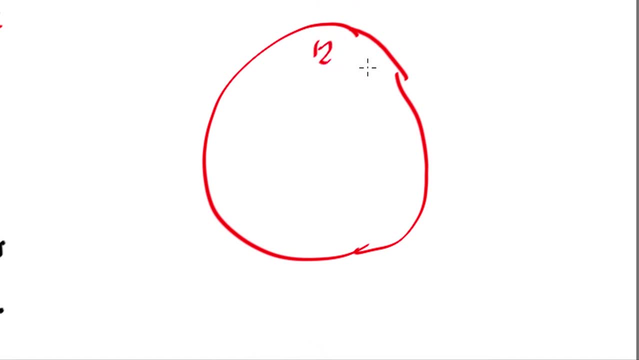 Okay, And then we know that this is 12. here We have 1,, 2,, 3,, 4.. 4,, 5,, 6,, 7, we have 8. here we have 9,, 10, and 11.. 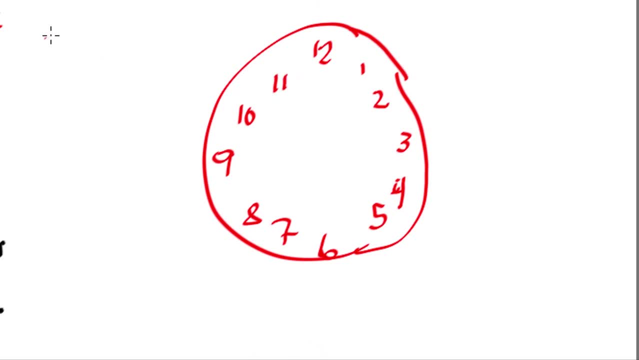 Now all the numbers here are in mod 12.. Modulo 12.. They are in modulo 12.. Why are they in modulo 12? Because after 12, we go back to 1.. Okay Right, There's no 13 o'clock. 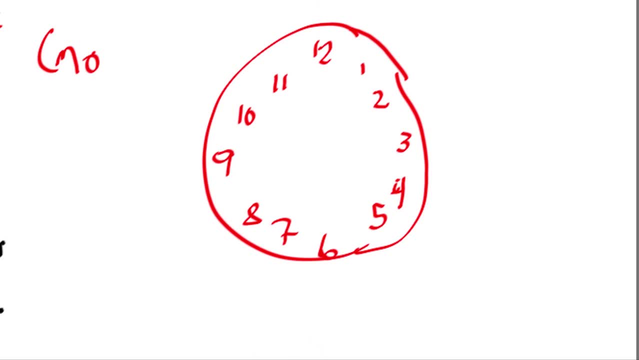 Unless, Unless, it's military time, Right, Unless it's military time. So you know, By the way, military time goes back to 0, 0.. That is, they are modulo 24,, by the way, Okay. 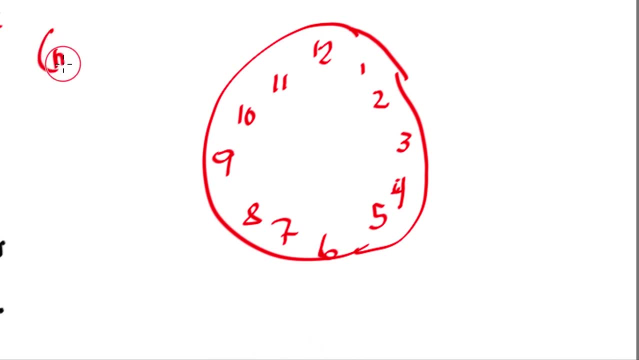 But let's use the normal way of reading clocks, So we're going to use mod 12 for that. Okay, So we know that after 12, there's 13.. Where is 13?? 13 is over here. 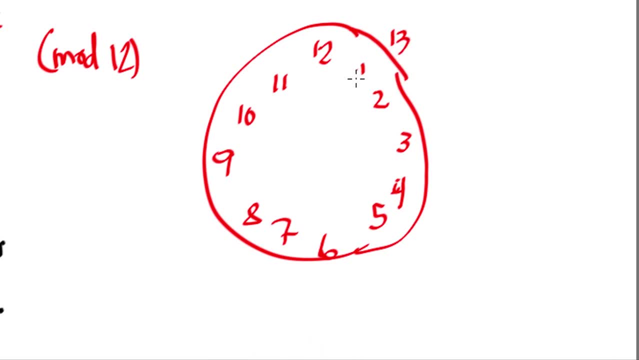 So when it's 13 o'clock in military time, we know that it's 1 o'clock. Okay, 14 is here, 15 is here, 16. 17., 18., 19., 20. 21.. 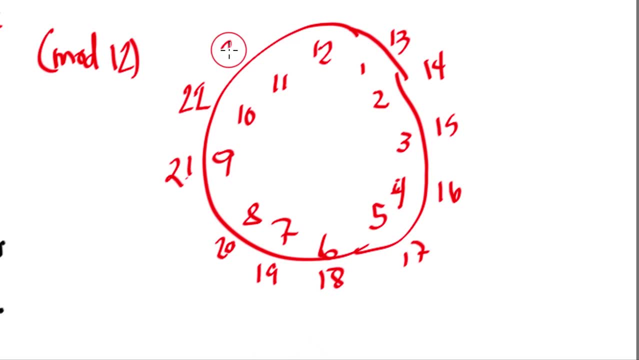 22., 23., 24. And then after that we go back to 25.. 25 will be on the 13th. Okay, 25 will be on the 13th. So, continuing in this manner, Let's have 24 here. 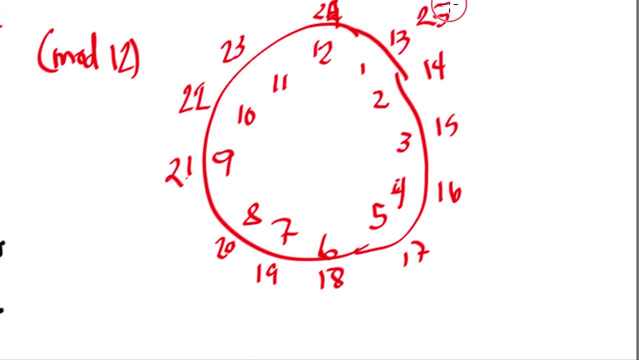 25 will be here, And then I think you can imagine so on. You can imagine this. Okay, Likewise, we can go back in reverse. 0 is over here, Because we're going to go back here. Negative 1 is here. 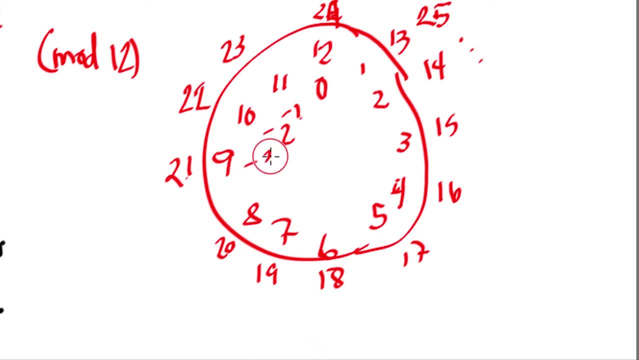 Negative 2 is here, Negative 3.. Negative 4 and so on. Okay, So we can say that in mod 12, we can say that Let's try to have some, Let's try to think this equivalence class. 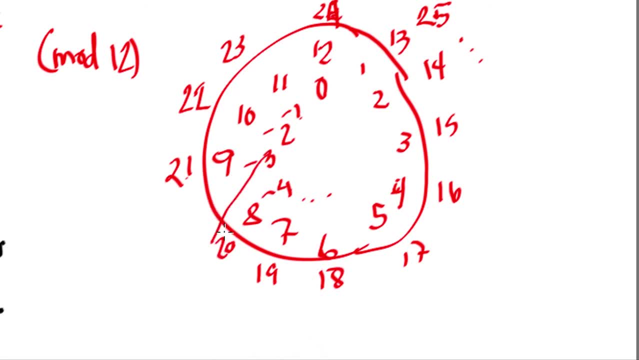 This one. Try to imagine this equivalence class And let's verify if they are indeed true by the statement of our definition. This one: Okay, Let's encircle this. It's quite difficult to encircle this one, Okay, So this one.